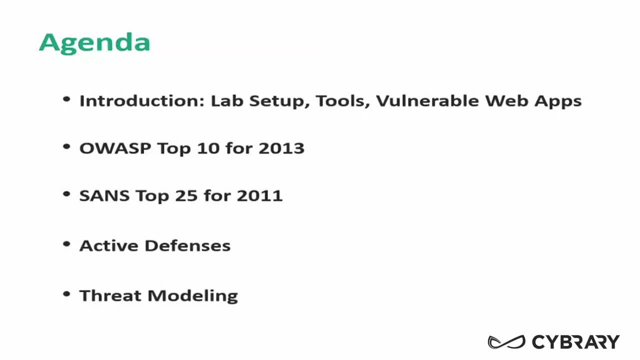 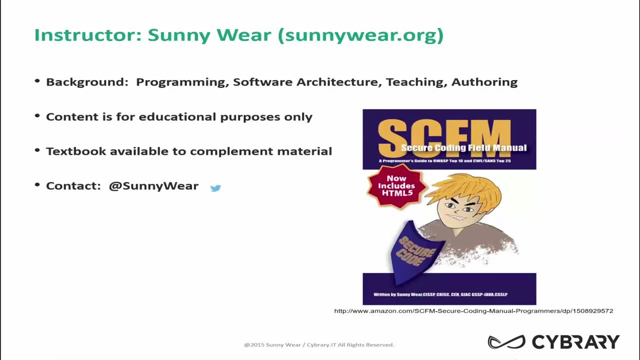 active defense techniques, and then we'll finish up the course with some threat modeling. Now first, just to let you know a little bit of background about myself. I come from a programming and architecture background. for over the past 20 years I also author several security books. 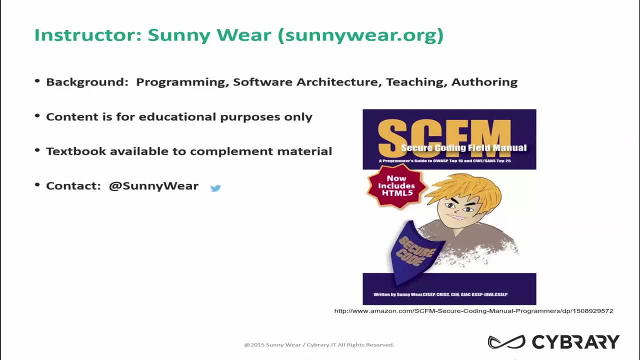 one of the books you could actually use as a textbook to complement the material that we're going to be going through in this class. The title of the book is Secure Coding Field Manual and it is available on Amazon. If you would like to contact me, you can reach me at my Twitter account at Sunny. 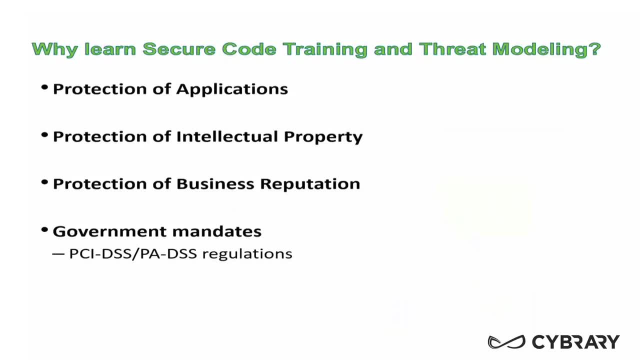 Witt. So why should we learn secure coding in the first place? Well, obviously we know that we need to protect our applications, which of course contains our intellectual property, and there are many, many reasons why we can get into protecting those applications, Anything from business reputation to basically making sure that our company stays in business so we have our jobs. 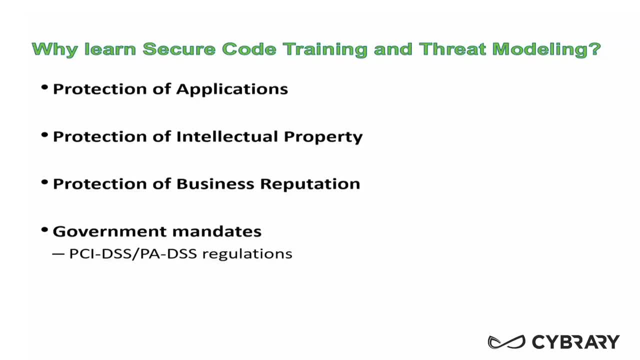 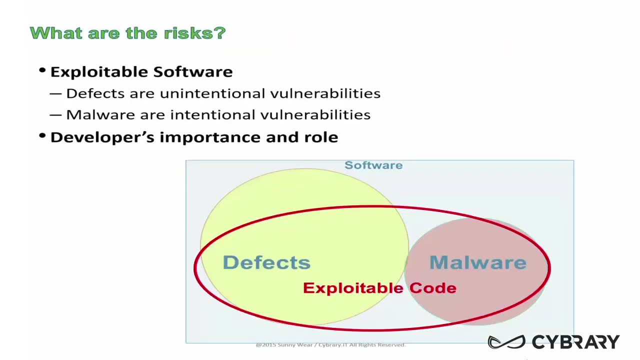 And then, of course, there are government mandates and particular regulations that are now requiring organizations to provide secure code training to their developers. So what exactly are the risks that we're trying to address as we cover this material? Mainly, in a nutshell, we're trying to address exploitable code. Now, exploitable code could be. 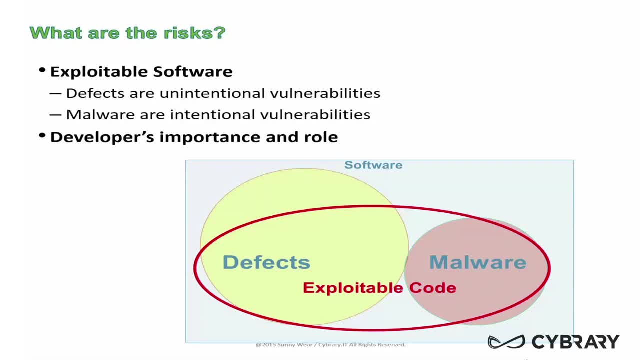 the result of various things. Two of the main areas would be defects or malware. Obviously, defects are unintended. These are programming bugs that programmers do and inadvertently create exposure points inside of their code. And then, of course, malware would be that intentional vulnerability, something injected into the code to make it exploitable. So what exactly are we going to? 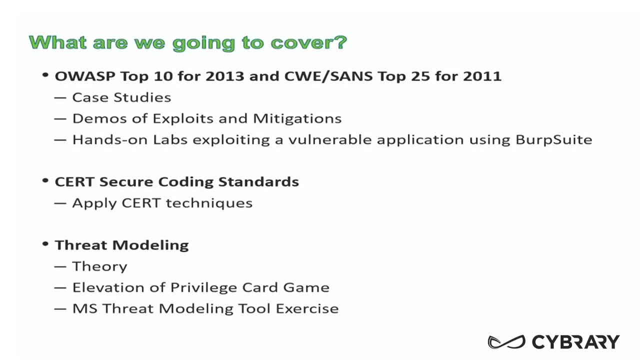 cover. We will cover the OWASP top 10 for 2013.. We will also cover the CWE SANS top 25 for 2011.. Now, as we go through each section, there will be case studies that we'll talk about Also. there's 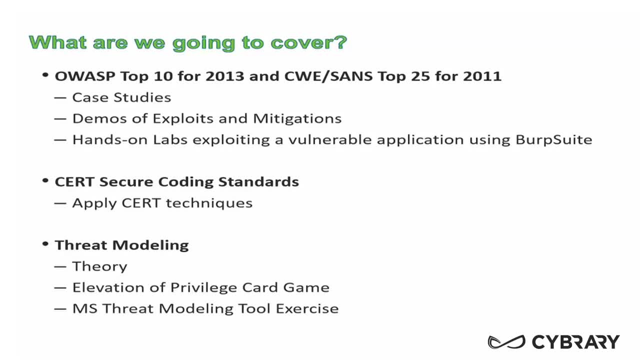 going to be lots of demos of the exploits and mitigations. I'll try to show you some code for the mitigations as we go through each section. So let's get started And then each module will have a hands-on lab where you actually need to perform the exploit. 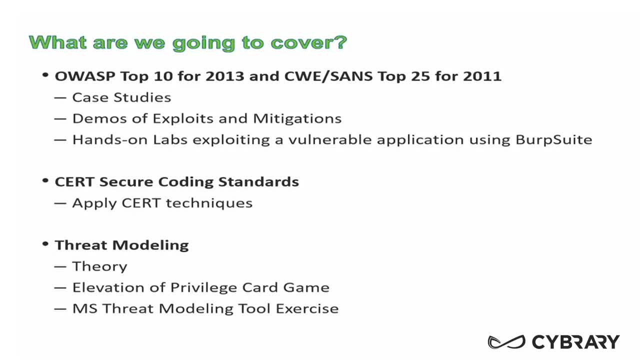 against a vulnerable web application. Now we might be using burp suite quite a bit. There are also some browser embedded plugins that we'll be using or that you can use if you feel more comfortable. Also, we're going to cover some of these cert secure coding standards. Now there are 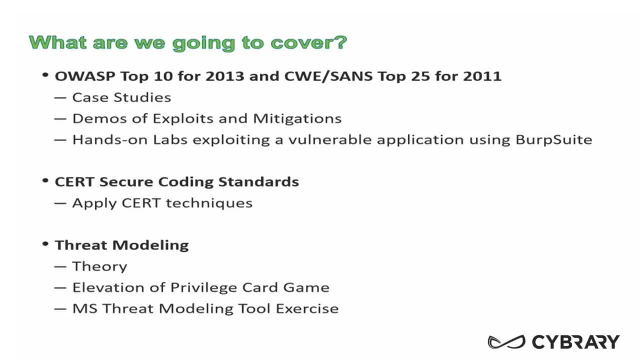 a couple of things that we're going to cover today. First of all, we're going to cover some of the problems of these, And so I've only picked out a handful to sprinkle in with our material, basically to provide some additional clarification, And then we'll go into some threat modeling. 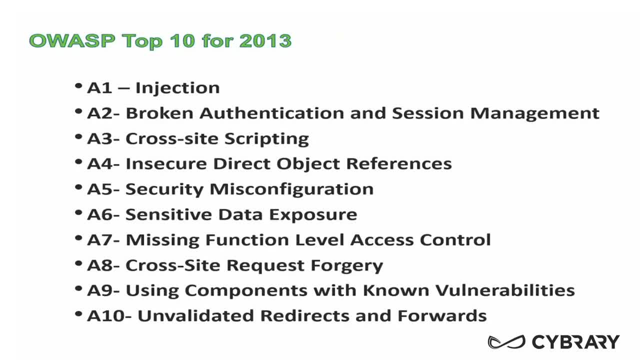 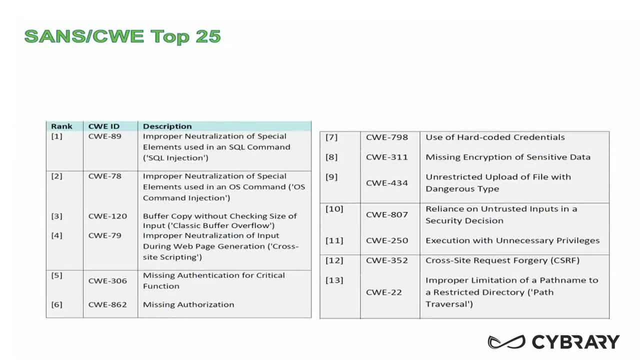 So the OWASP top 10 for 2013,. we're going to go through this list extensively. And then the SANS CWE top 25, basically, we are going to cover all of the categories that are not previously covered in the OWASP. 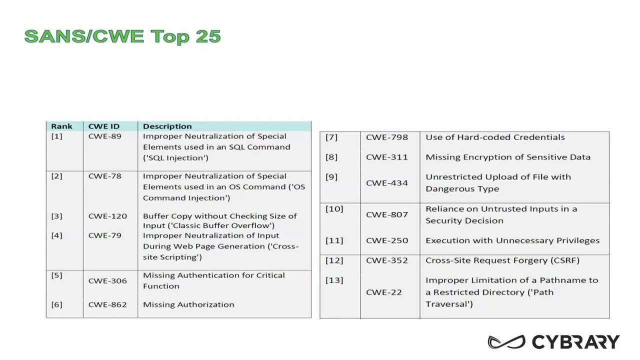 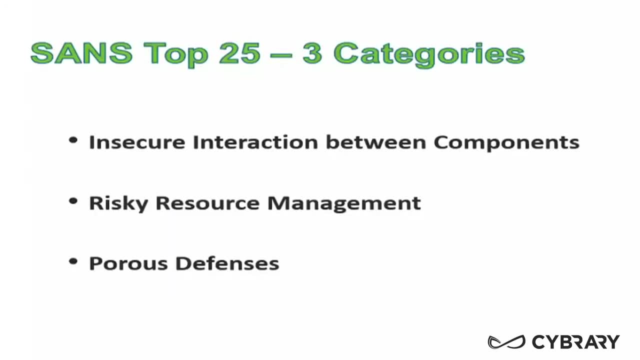 section. So I'm listing them out here for your viewing, but realize we'll go into each one of these in depth in our material. Now there are three main categories that I've broken the material up for the SANS top 25 into. 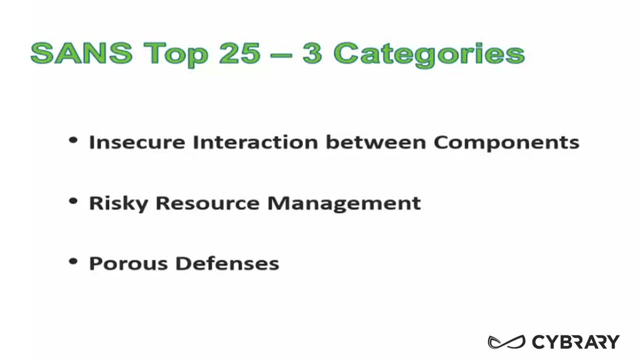 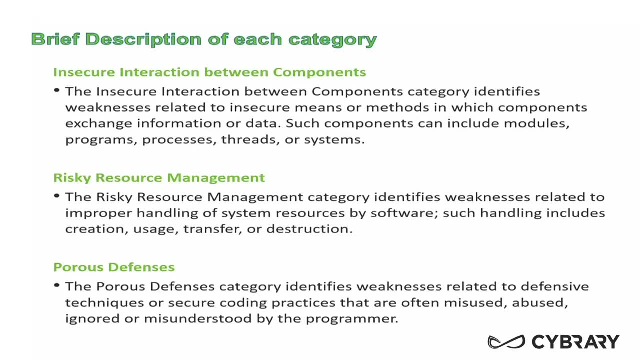 The categories include insecure interaction between components, risky resource management and porous defenses. If we were to take a look at a definition for each one of those, we can see that the riskier the interaction between components is exactly that: where you've got some sort of weakness. 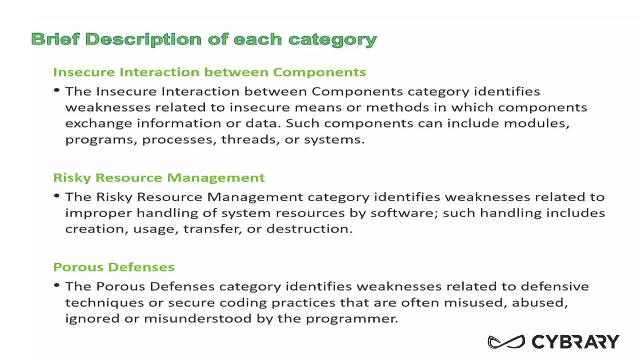 that can occur during the exchange of information or data or in the interaction of components or modules or programs together. Risky resource management has to do with the handling of your system resources and some sort of weak or risky manner Now porous defenses. this is where we have. 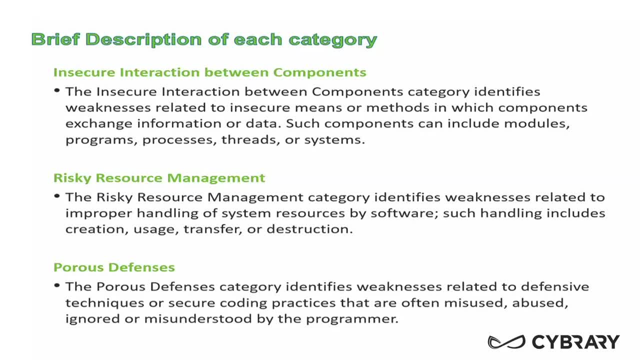 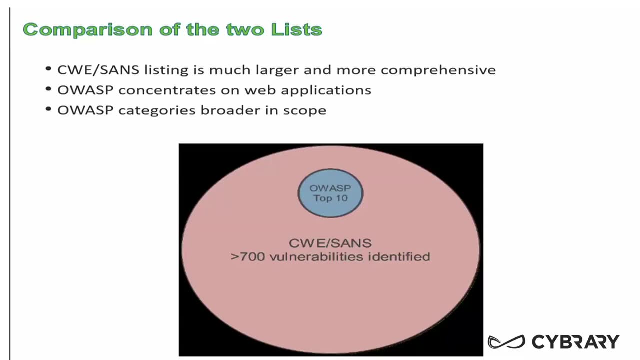 some kind of like a problem. So we're going to go through this list of five. The most common mistake we see is that the software errors are not correctly identified with the program. Most of the time the programers are misidentified. If you were to try to compare the two lists together, you would realize just how huge the CWESANS listing is. They have over 700 vulnerabilities or software errors identified. The OWASP is just a very small subset of those errors. If you were to compare the two lists together, you would realize just how huge the CWESANS listing is. The OWASP is just a very small subset of those errors.